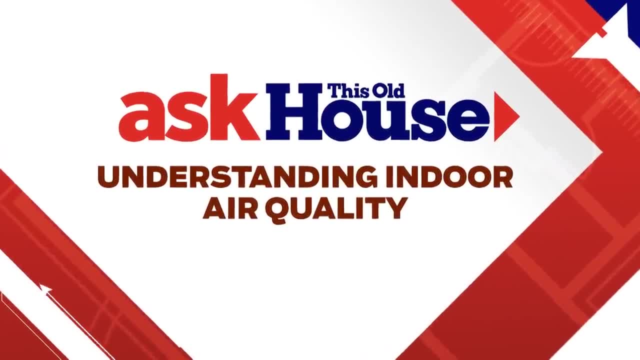 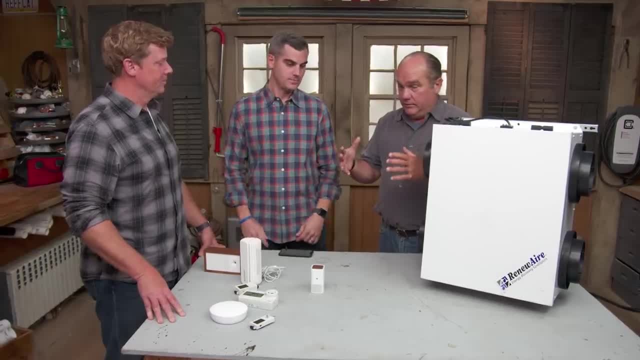 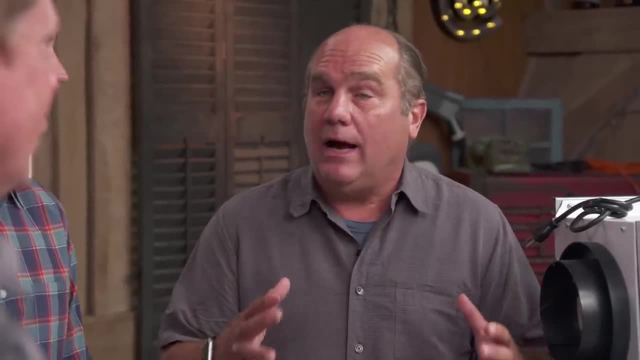 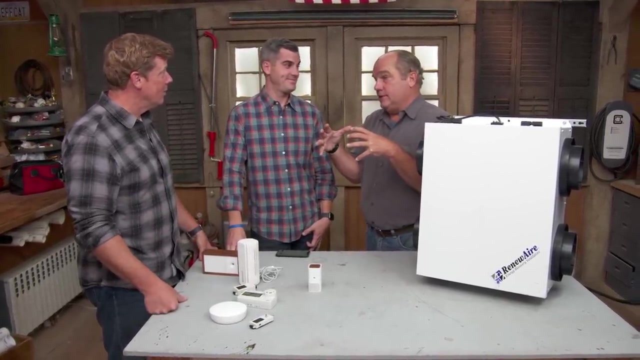 Hey Ross, hey Richard, Hey, What are you guys working on Talking about indoor air quality today? Cool, You know buildings need to breathe And when I first got in this business they breathed plenty. You know they breathed at a rate of 10 to 12 air changes per hour. That needs like a full stop to make people understand that, Like all of the air in the house leaves 10, 12 times an hour Right. 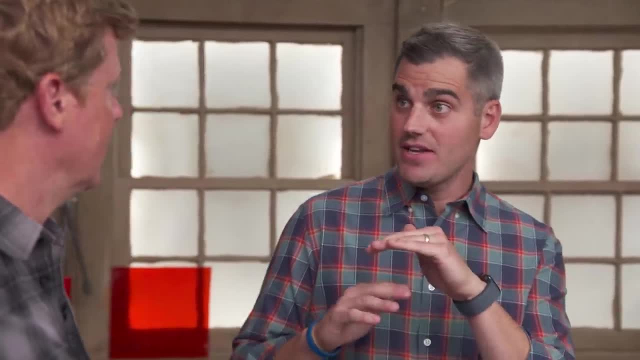 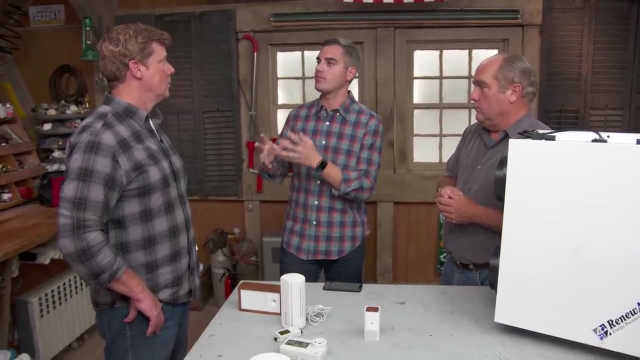 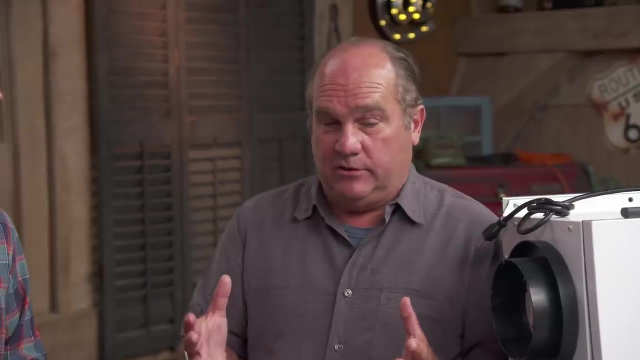 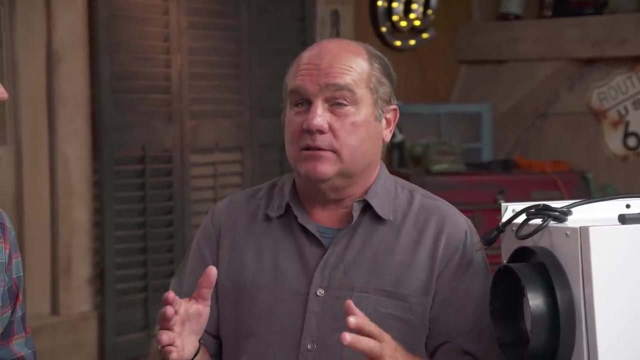 That's a lot of breathing. So nowadays, what are we seeing? Nationally, the average is seven air changes, And code in Massachusetts for new construction is three, And that's because of spray foam and air barriers. You know we're getting away from the traditional building materials we used to use. So how bad is the indoor air quality as a result? Inside this house it's the ultimate sort of petri dish, this hamper really, where stuff is trapped And people don't realize that the air inside most houses is two to five times worse than any air you're going to find on a busy city street. 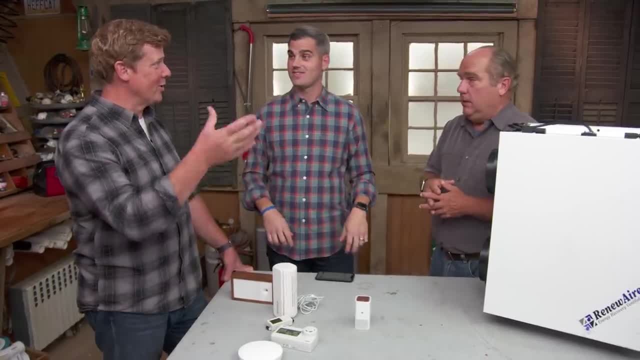 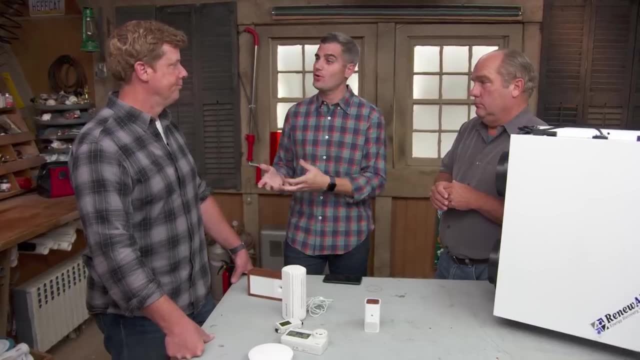 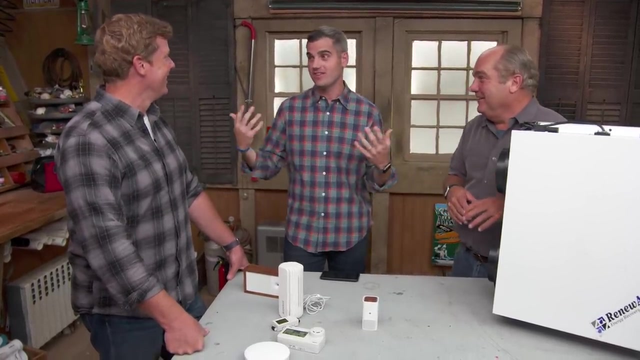 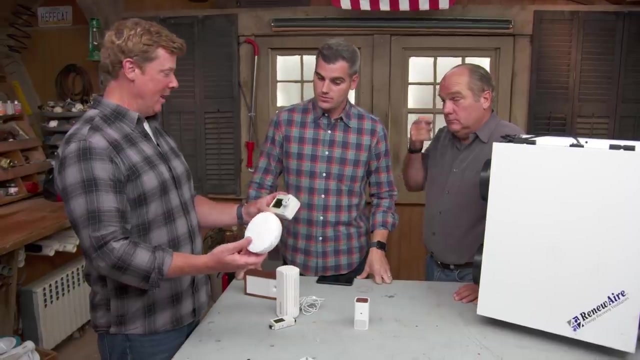 Because it's trapped. That's depressing, Absolutely. Indoor air is dirtier than outdoor air, Absolutely. And these pollutants are coming from everywhere. The cleaning products under our sink, paints, carpets, furniture- I mean cooking People Right me, You- I talk a lot, You A lot- The gas range, the oven, right Those are all giving off chemicals. So these gadgets that I'm looking at here, are they going to tell me what I've got in the air and how bad it is? So these are a variety of different monitors that have different sensors, So this one does CO2.. 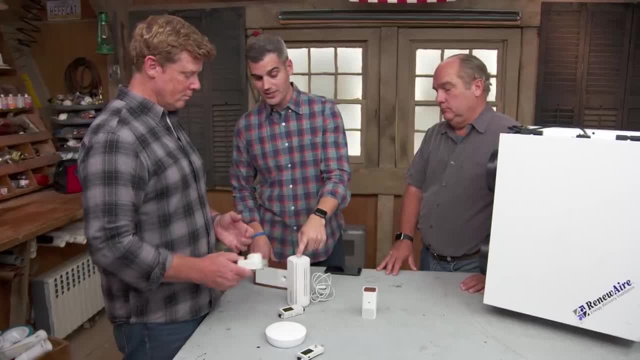 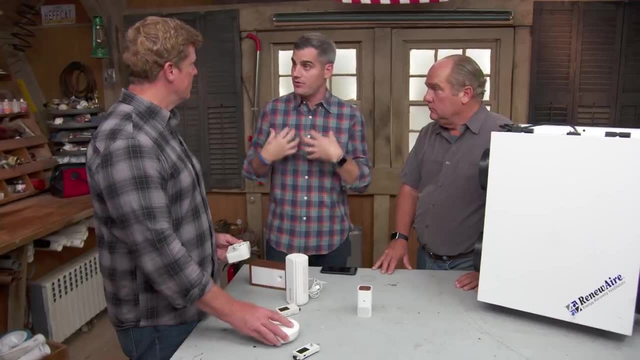 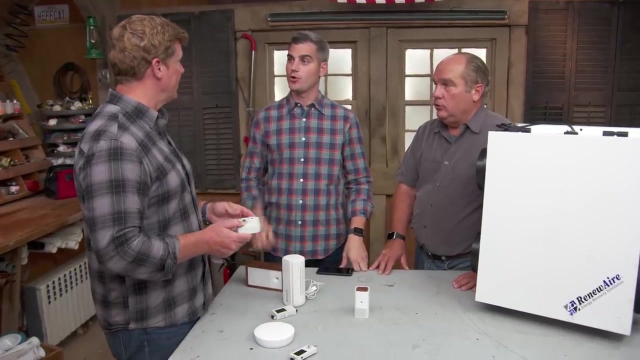 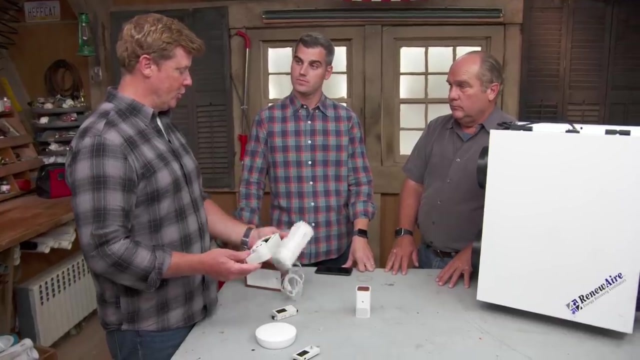 Right Where we're breathing out. it does temperature, it does relative humidity. This one, for example, is doing VOCs, particulate matter. Those are the particulates that are really really small, You can't see, that you can actually inhale, get into your lungs and into your bloodstream. So we don't have a device that tells us everything that's in the air and breaks it down. You need a device to go looking for a particular thing. You're picking specific things. You've got to decide what you want to monitor and find the right device for it. So once this thing tells me I have too much CO2 or what was it? VOCs, VOCs or particulate matter- What do I do with it? Well, you've got to ventilate. You know a building needs to be ventilated. 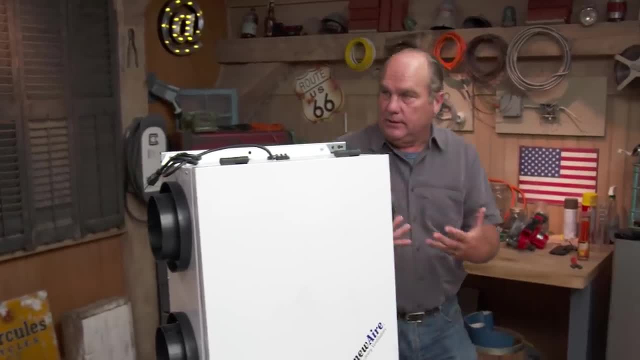 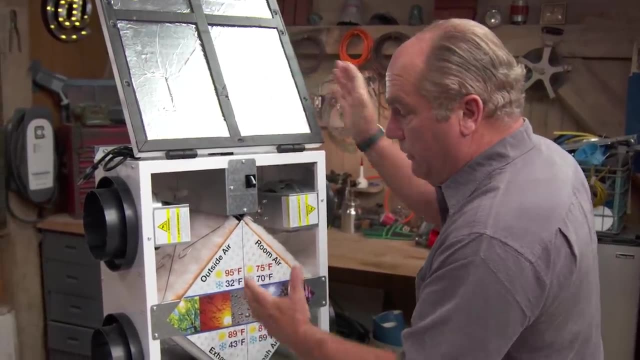 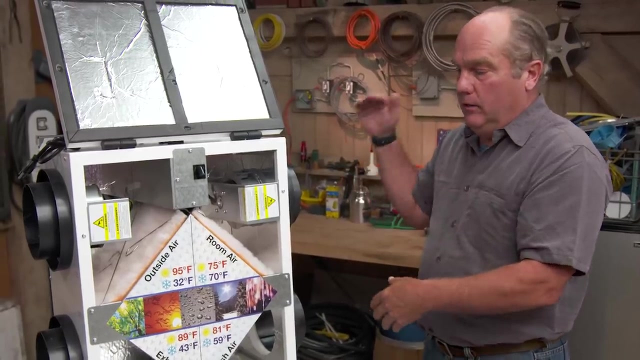 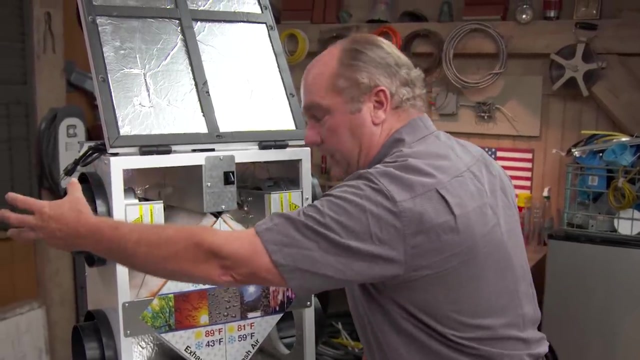 It doesn't need to breathe. but it doesn't need to breathe through every door and window. It needs to have a set of lungs. And if I was talking about a set of lungs it would be a box, something like this, either called an HRV or an ERV. So how it works is that you've got this core in the middle and now stale air that would leave the building from bathrooms or contaminated air, would pass this way with a fan across this core and to outside. But at the very same time another fan brings exhaust outside air in across this core in the opposing direction. So imagine this here in the winter. 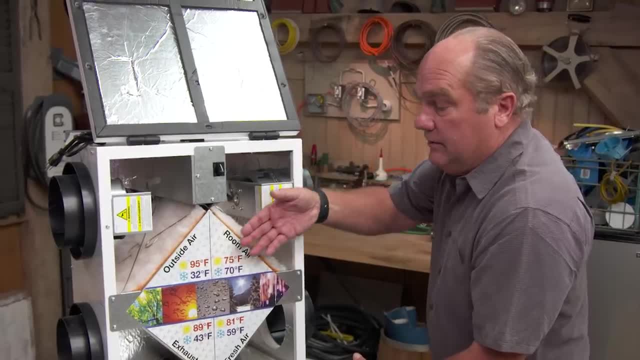 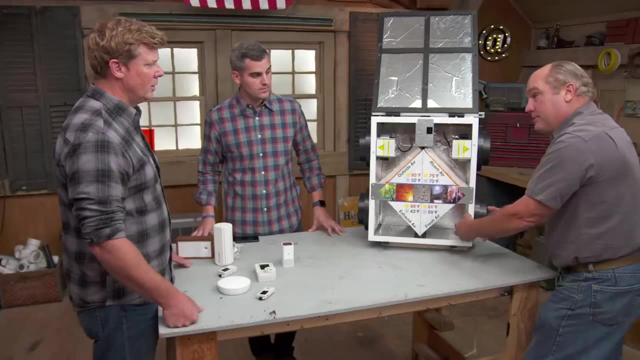 Right, It's rich with temperature and it goes, wants to leave to outside. It would have just gone outside. Now the cold air picks up the heat that's in the exiting air and it keeps the energy inside the building. So you keep the energy inside the building but exhaust the fresh air, exhaust the stale air out of the building. 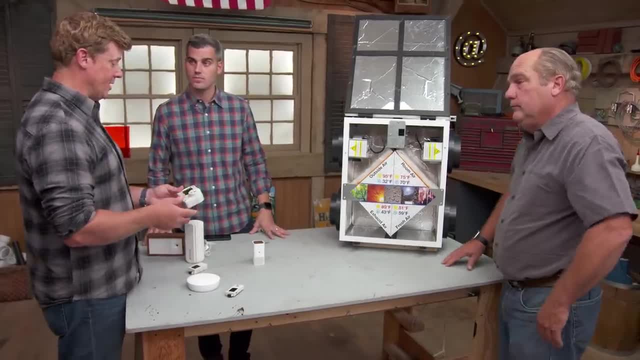 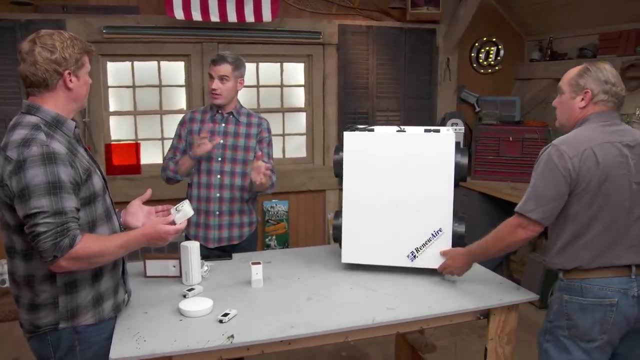 We've seen those. before I get it. I put one of these things on my wall which I have not seen before. What does it do? Does it beep and say turn on or alarm, or So yeah, some of them will just give you a visual indicator, like a light right that changes colors. Some of them will actually talk to your phone. 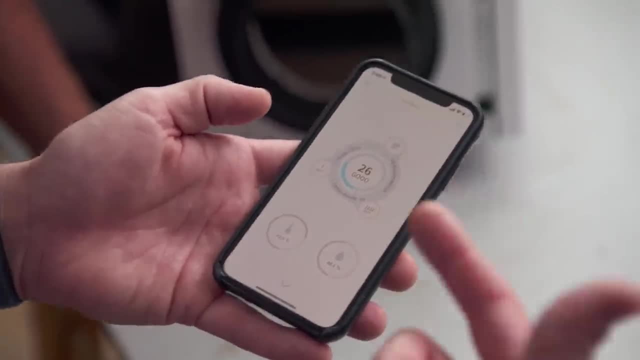 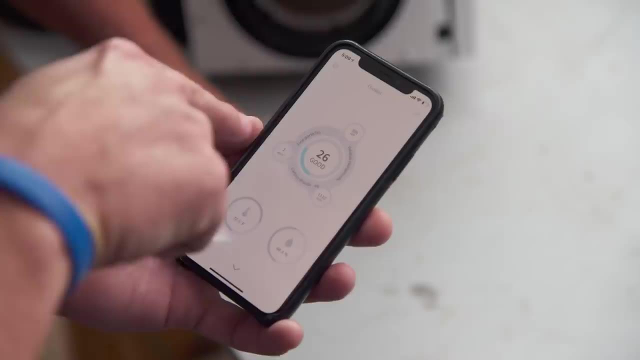 So it'll actually send you a notification or it'll actually give you a graph that shows you when you actually have bad air quality, And so here's a main screen for one of them. I can see three different pollutants: particulate matter, VOCs and carbon dioxide. I can also see temperature and relative humidity in the space. 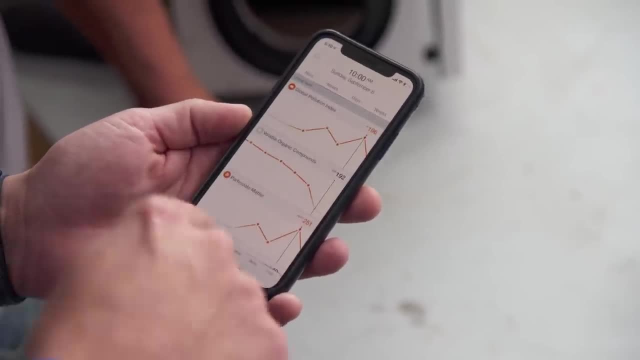 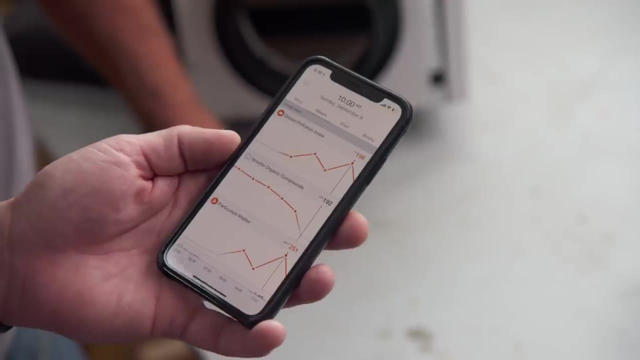 And here I'm actually seeing them over time. So here's an event where our particulate matter actually spiked to 251. Caused by- And that was caused by- the gas range being on without the exhaust fan running. Oh, interesting, Okay. 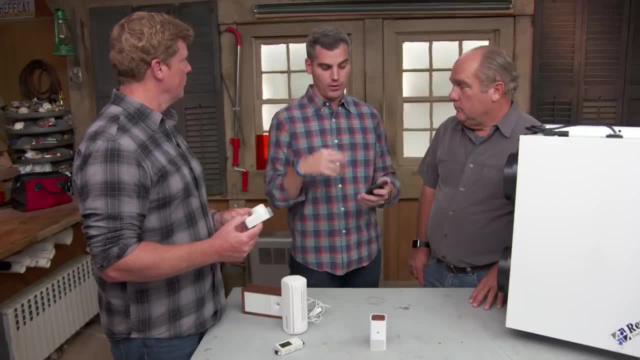 At the most basic level, you could crack a window or run an exhaust fan when you see this, but where it's going is that these devices now are talking to these devices or other exhaust fans Like a smart thermostat. That's right. Now we've got smart air. 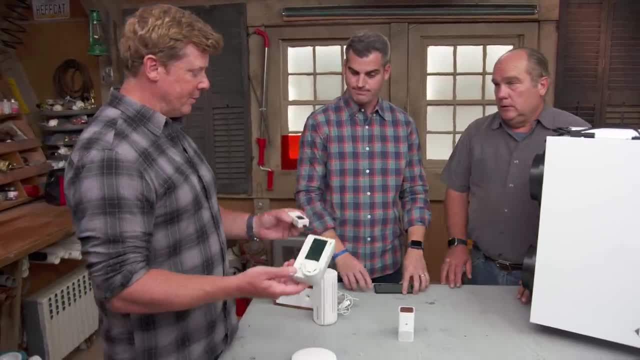 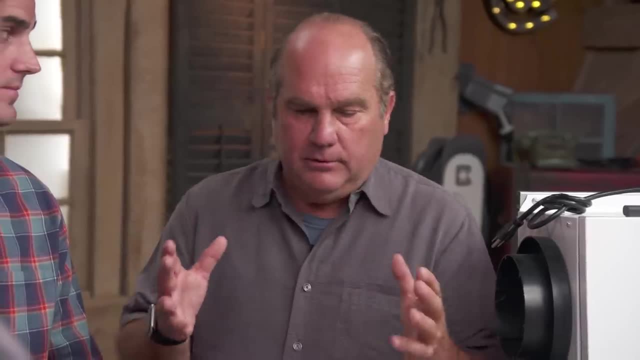 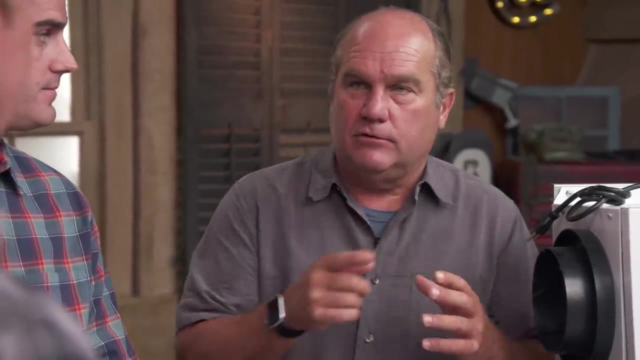 So it does it automatically behind the scenes. So what do you guys think New, normal? Are we going to be seeing a lot of these? I think you have to. Everybody's going to watch it. The buildings are only getting tighter, And the last thing I'll say about this is I built a new house- what? 15 years ago? super tight, with all the foam insulation, tight windows, and I didn't have one of these for the first year. 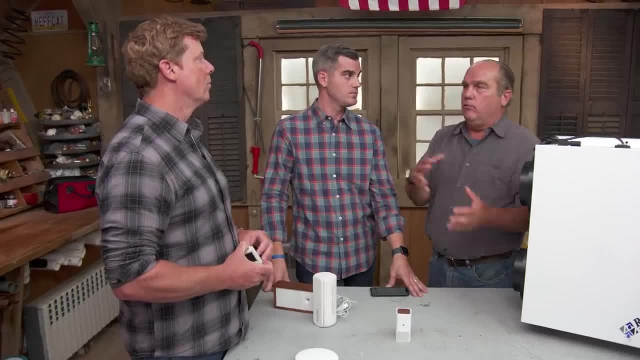 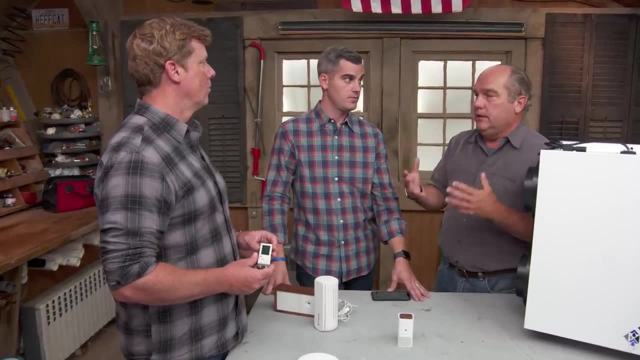 And what happened is we always felt Sluggish And mold formed everywhere. And then we put it in and it just changed. It's an intangible that you can't really transfer until you live with it, Just to have fresh air in the building. it just changes the way you live in the space.